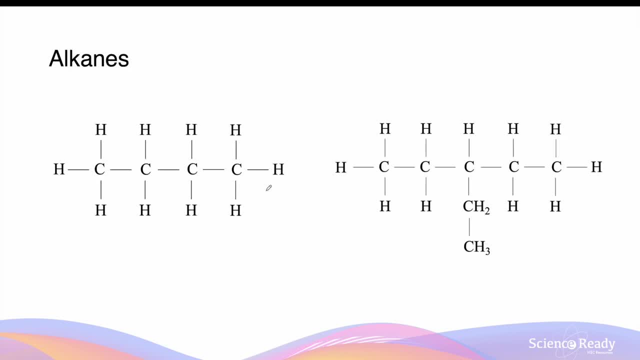 the priorities will affect the names Starting with alkanes. the names of alkanes will end with the suffix of a-n-e. When there are four consecutive carbons in the molecule of alkane, this is called butane, where the prefix bute represents the number four In this molecule. 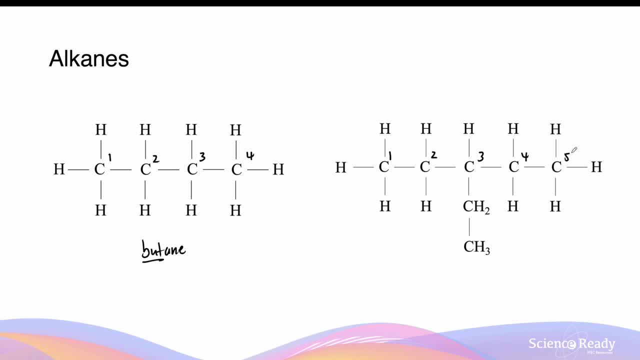 we can count one, two, three, four, five, Five consecutive carbons, and that leaves behind two carbon atoms in an ethyl group. So the name of this molecule is butane. The name of this molecule will end with the suffix pentane. 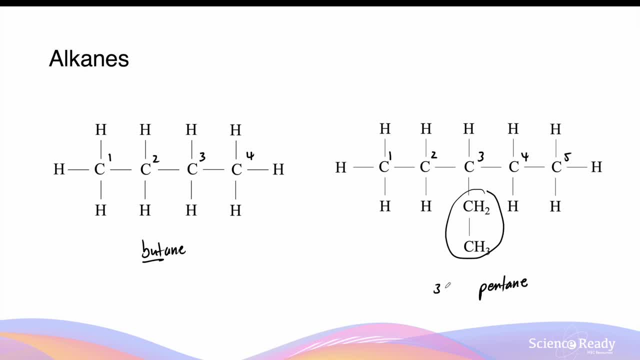 and the ethyl group is on the third carbon, so therefore this is called 3-ethyl-pentane Alkanes are hydrocarbons that contain a double bond between carbon atoms. In most cases you will have to denote the position of the double bond In this molecule of alkane, the double bond. 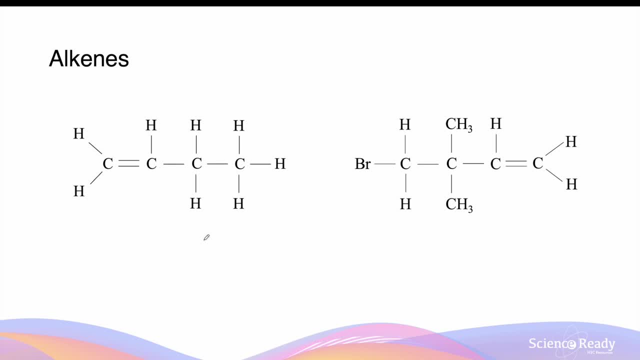 is in the first of the three positions. Therefore, this is called Bute's winding. Remember that we always should count the carbon chain in such a way so that the functional group receives the lowest number possible. This is the reason why this is But-1-ing instead of But-3-ing. 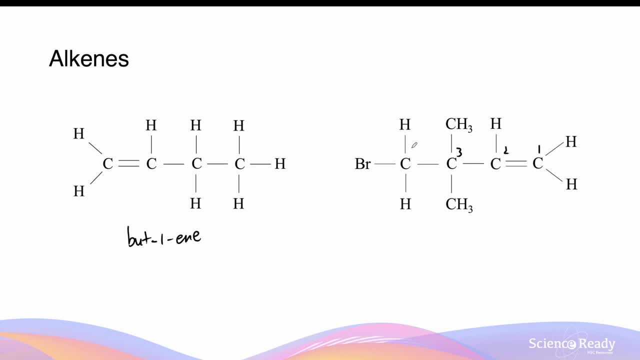 In this molecule we can count one, two, three, four consecutive carbons, and the double bond lies in the first bond position, So this is again But-1-ing. In addition to the butane chain, there are two methyl groups that lie on the third carbon and there's one, bromine. 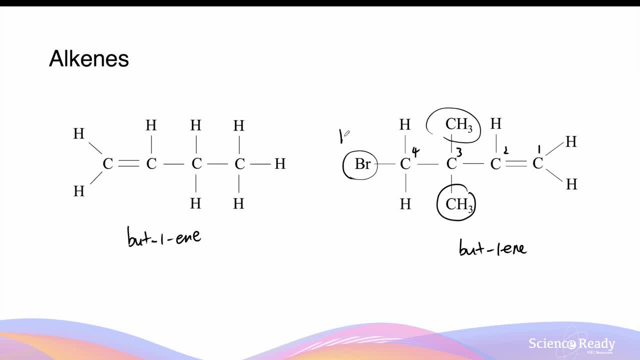 substituent. on the fourth, carbon Bromine is denoted by the prefix bromo, whereas the methyl groups are, of course, denoted by the word methyl. When there are multiple substituents or branches in the molecule, you need to write the names of the branches in alphabetical order, So this will. 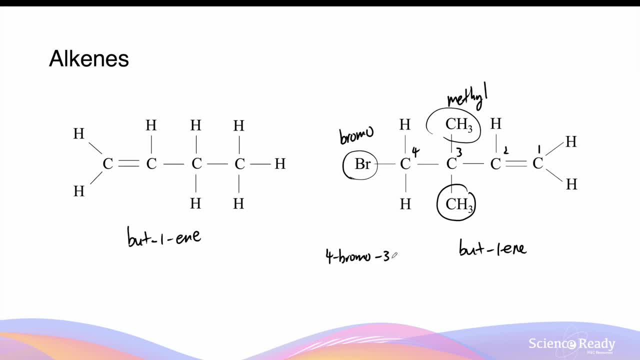 be 4-bromo, and there are two methyl groups on the third carbon, so it'll be 3-3-dimethyl-but-1-ene. Just a side note: the prefix di denoting the presence of two methyl groups is not considered. 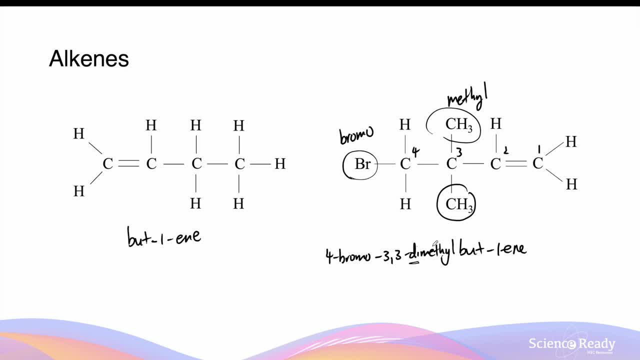 when you're arranging the branches in alphabetical order. Alkynes are hydrocarbons with triple bonds between carbon atoms. In this case there are 1,, 2,, 3,, 4, 5 consecutive carbon atoms and a triple bond lies in the first bond position, So this will be called pent-1-ime. 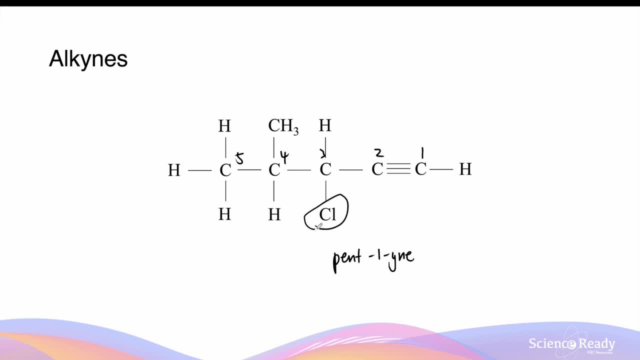 In addition to the main carbon chain, you have a chlorine group, which is represented by the word chloro, and a methyl group on the fourth carbon. Since chloro c comes before methyl, we'll write chloro first, So this is called 3-chloro-4-methyl-pent-1-ime. 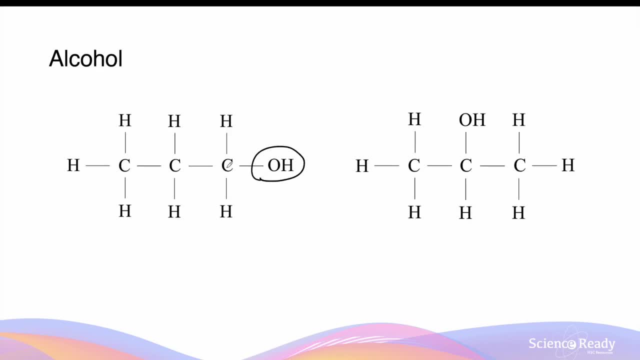 Alcohols are molecules with an OH group on a carbon atom that only has hydrogen and carbon single bonds. The presence of alcohols is denoted by the suffix ol. In the first example of alcohols there's one, two, three consecutive carbon atoms. This molecule will be called pro- and 1-ol, The prefix prop. 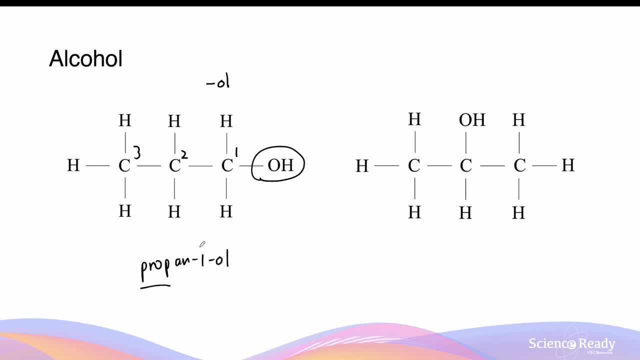 represents three consecutive carbons and since the alcohol is in the first carbon, this is denoted by one. Propan-1-ol is a primary alcohol, because the carbon atom that is connected to the alcohol group is only next to one other carbon atom. In this molecule. there's again three consecutive. 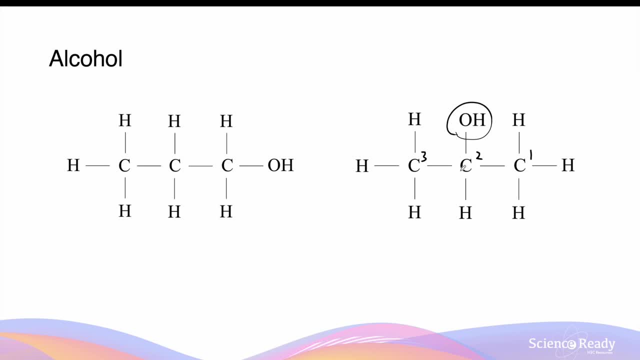 carbon atoms, but now, this time the alcohol functional group is only next to one other carbon atom. The name of this molecule is propan-2-ol. Propan-2-ol is later classified as a secondary alcohol because the carbon atom that's 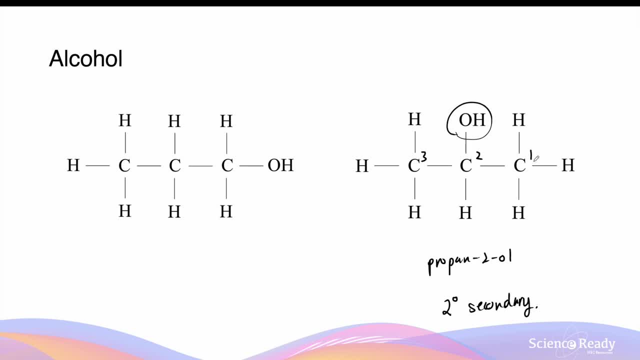 connected to the alcohol group is next to two other adjacent carbon atoms. In this molecule of alcohol groups there are also three consecutive carbon atoms. The name of the alcohol group is propan-2-ol, And the alcohol group also comes with two capitides. which, for many of you may know, may function as ninguna. Propan-2-ol is classified as a secondary carbon atom, And this, too, is how a carbon carbon group is, BECAUSE the carbon group is facilities known for oil and the adjuvant of CO2, which is P- такой好. 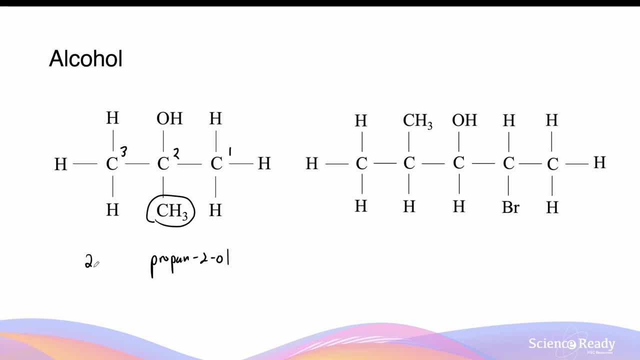 the carbon group is attached to the compassionate carbon group which is propan, because, I repeat, second carbon atom. Proban-2-ol is also second carbon atom because the carbon group is next to, while there is ne group attached to the second carbon. so we'll write this as 2-methyl-propanolol. This is 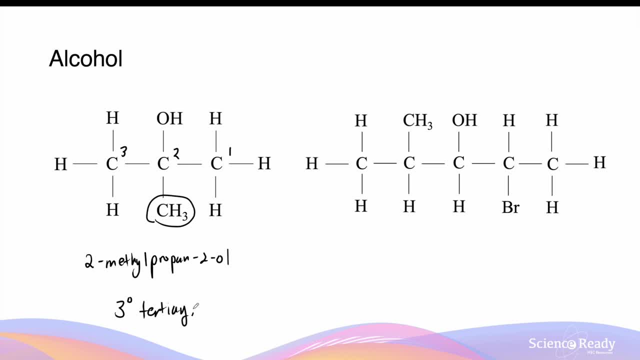 classified as a tertiary alcohol because the carbon atom that is bonded to the alcohol is adjacent to three other carbon atoms. In this molecule of alcohol there's one, two, three, four, five consecutive carbon atoms, and the main alcohol functional group is attached to the third. 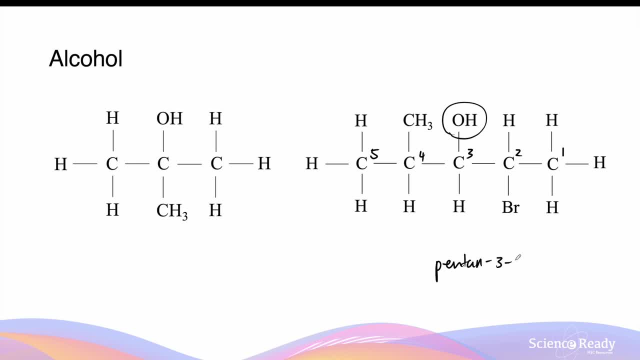 carbon atom. This will be called pentan-3-ol. The presence of bromine is denoted by bromo and the presence of a carbon hydrogen is noted by methyl. Since B comes before M in the alphabet, we'll write bromo first, which is 2-bromo 4-methyl-pentan-3-ol. Sometimes in a molecule there can be more than 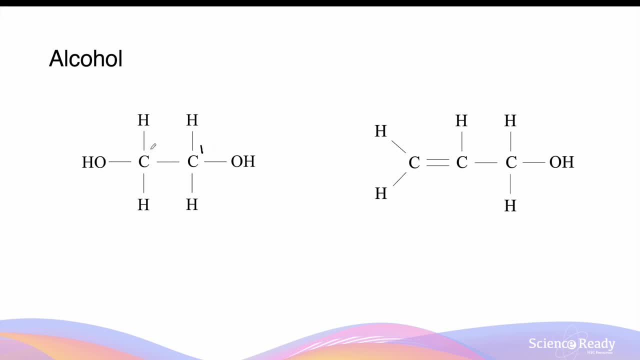 one alcohol functional group. In this case there are two carbon atoms, so this would be called ethan one. two diol Diol here refers to the presence of two alcohol functional groups. Sometimes the alcohol functional group can be also present alongside an alkene functional group. 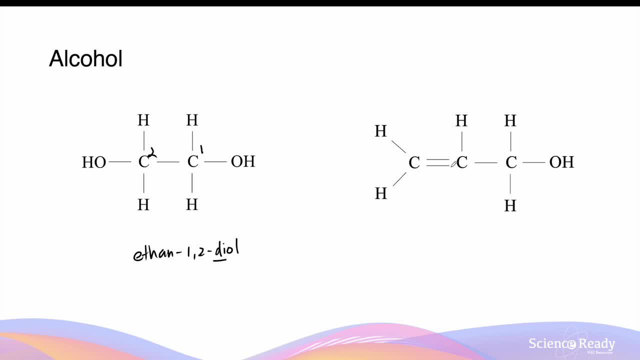 Now recall that alcohols have higher priority than alkenes, so we need to give the alcohol the lower number compared to the alkene. As a result, we'll be counting the carbon atom from right to left: one, two, three. There are three consecutive carbon atoms, so this will be called: 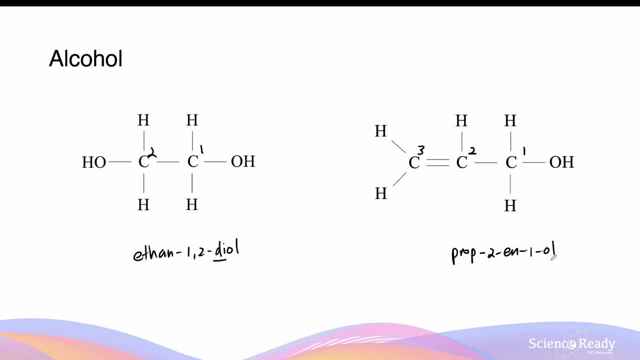 propan-2-methyl-propanolol. The double bond is in the second bond position between the second and third carbon atom, and the alcohol is attached to the first carbon atom. In organic chemistry there are a group of organic molecules known as carbonyl compounds. 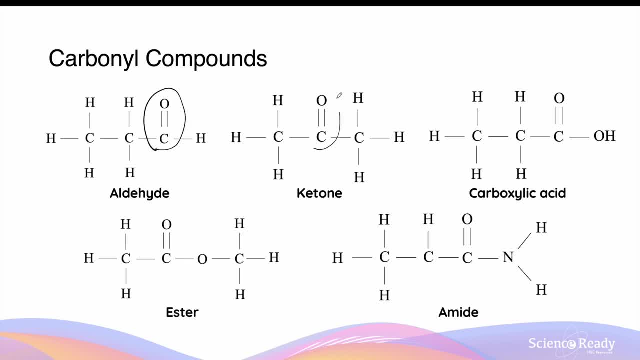 These functional groups all contain a carbon to oxygen double bond. as I'm circling around here, This bond is called a carbonyl bond. Typically, we refer to the carbon atom that has a double bond of oxygen, as the carbonyl carbon In aldehyde. the carbonyl carbon is between a carbon atom and a hydrogen. 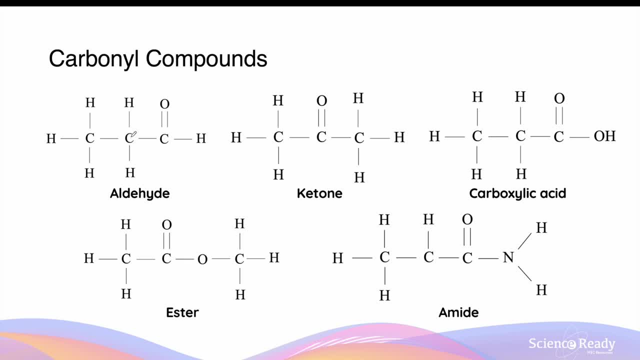 in a ketone. the carbon node at the carbon atom is between two other carbon atoms and in carboxylic acid the car is attached to another carbon atom instead of a hydrogen that we will see in carboxylic acid. In an amide functional group, the carbonyl carbon is next to a carbon atom and a nitrogen atom. 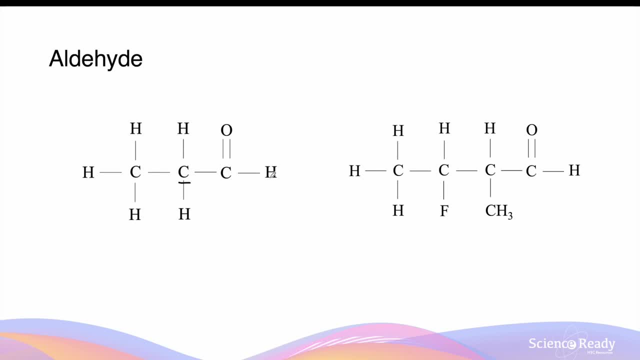 In an aldehyde, the carbonyl carbon is between a carbon atom and a hydrogen atom. The suffix of an aldehyde ends with "-al". The way you can remember this is that the beginning of aldehyde is also such as "-al". In the first molecule there are three concentric carbon atoms. 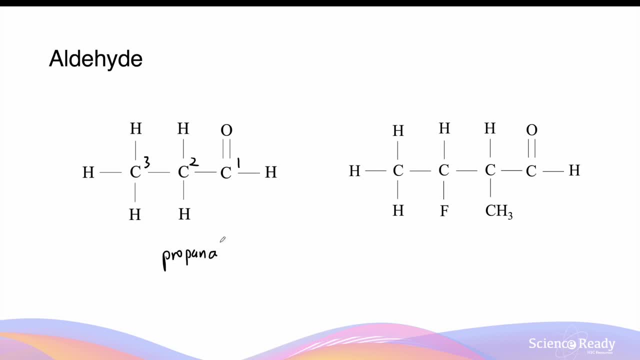 Therefore the name of this molecule is propan-al, Because an aldehyde functional group is always at the end of the molecule. we do not need to number the position of the aldehyde functional group because we assume that it's always on the first carbon atom. 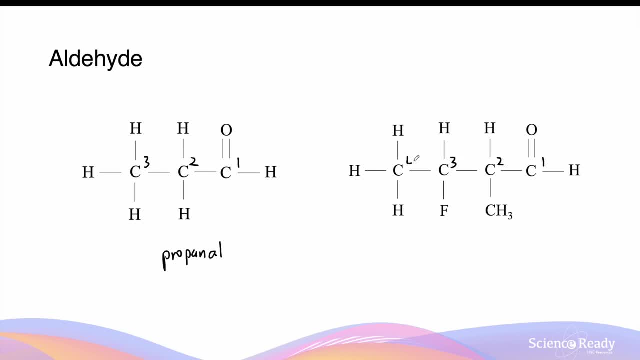 In the second molecule there are one, two, three, four consecutive carbon atoms, And again the aldehyde will be presumed to be on the first carbon. So the name of this molecule is butan-al, without any numbers, And in addition there's a methyl group on the second carbon atom and a 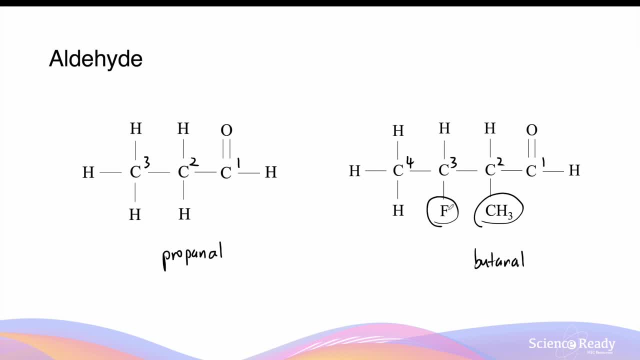 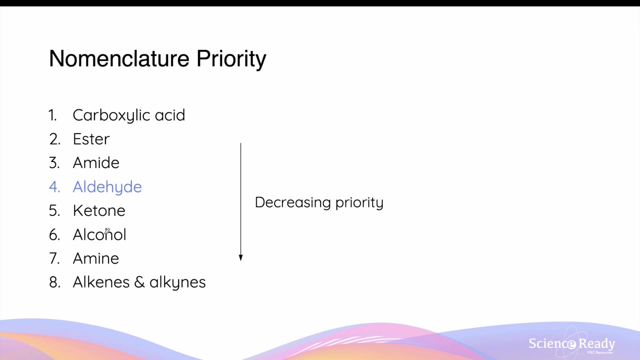 fluorine atom on the third carbon atom. Since fluoro comes from the M, we'll write down three fluoro before the methyl Three fluoro. two methyl butan-al Aldehydes have higher priority than ketones, alcohols, amines and alkenes and alkynes. 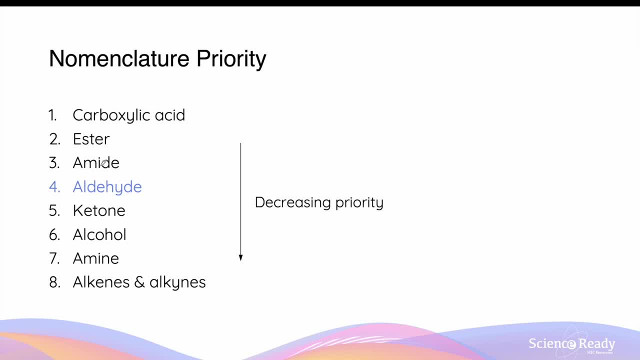 but lower priority than carboxylic acids, esters and amides. In the molecule containing an alcohol and aldehyde, the suffix will be given to the higher priority aldehyde group and therefore the alcohol will be named using its prefix, which is called hydroxy. Therefore the name 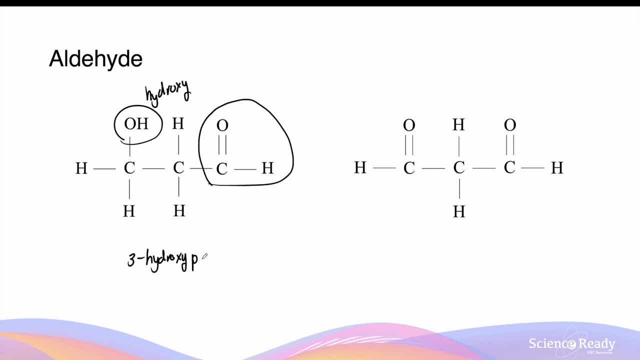 of this molecule is 3-hydroxy-propan-L. In a molecule containing two aldehyde functional groups, we can denote this by writing propan-di-L. The letters di denotes the presence of two aldehyde functional groups. A ketone functional group is where the carbon or carbon is sandwiched. 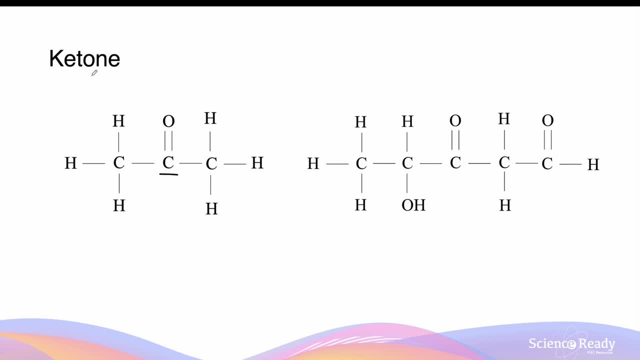 between two other carbon atoms. The ending of a ketone is in its name: O-N-E-O. When there are three consented carbon atoms, this is called propan-NO. We don't need to use a number 2 to denote the position of the ketone functional group, because a ketone must have. 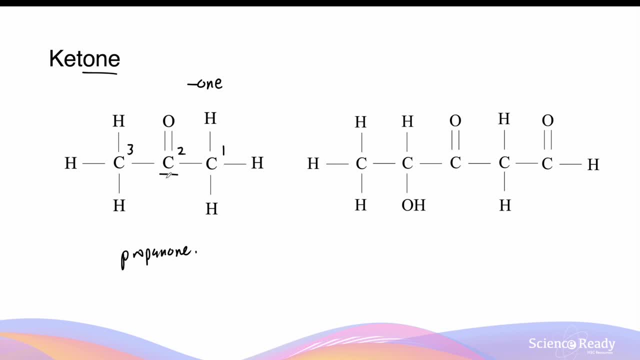 a minimum of three carbon atoms. So in other words, the ketone functional group can only be on the ketone functional group. In this molecule there are three different functional groups. There's an aldehyde, a ketone and an alcohol. Aldehydes have higher priority than ketones, which has higher priority. 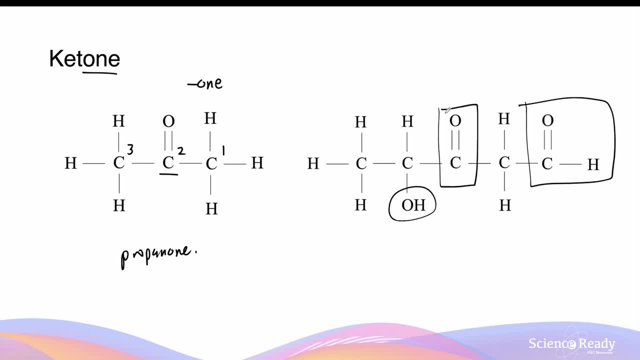 than an alcohol. So, in other words, the suffix for this molecule will be for the aldehyde, which will be A-L, and the presence of the ketone and alcohol will be denoted by the prefixes. The prefix for ketone is oxo and the prefix for alcohol is hydroxy. 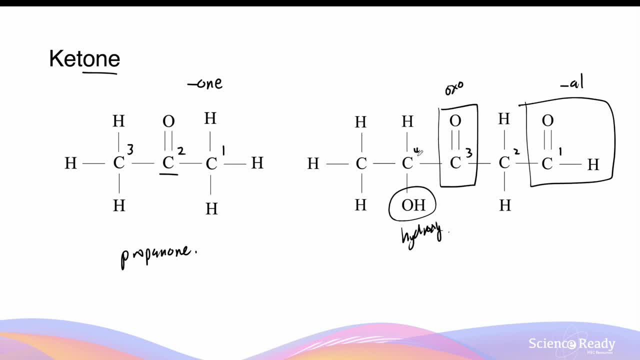 In this molecule there are 1,, 2,, 3,, 4, 5 consecutive carbon atoms, so the ending of this name will be pentan-L. Since H comes with an O on the alphabet, we'll write hydroxy first. 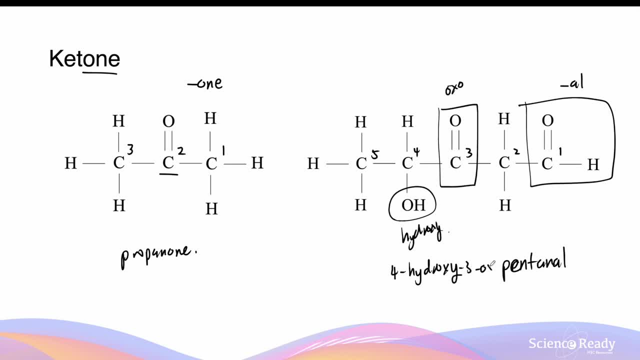 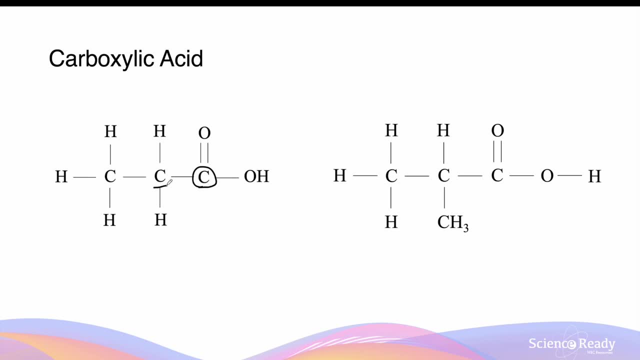 so this will be 4-hydroxy-3-oxo-pentan-L. Carboxylic acids are molecules where the carbonyl carbon is sandwiched between a carbon atom and an OH group, The suffix for carboxylic. 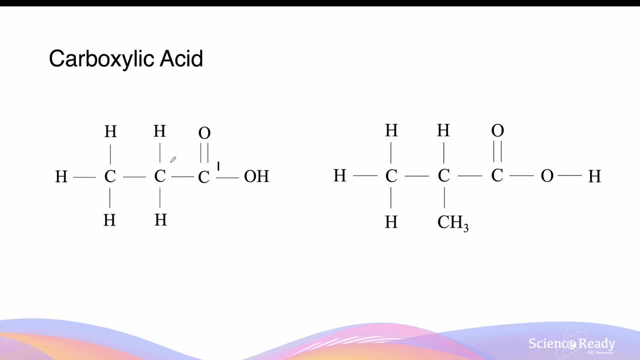 acid ends with oic-acid. In the first molecule there are 3 consecutive carbon atoms. therefore the name of this compound is propanoic acid. In the second molecule there are again 1,, 2, 3 carbon atoms, but there's a methyl group on the second carbon atom. Therefore, this 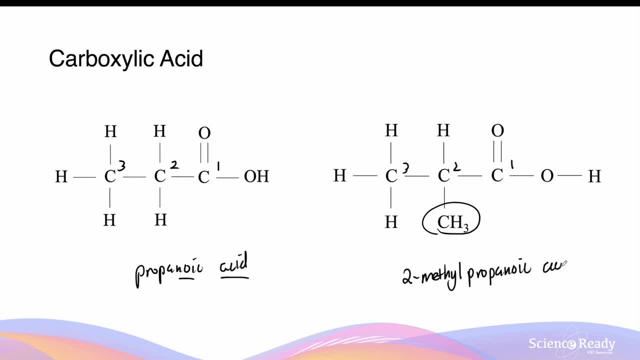 is called 2-methyl-propanoic acid, Since acids are proton donors. when carboxylic acids give away their proton, they form the conjugate base. In the third molecule there are 2-carboxylate ions, and this is where the OH group becomes. an oxygen with a negative charge. The suffix for carboxylate ions is oate. In the first molecule, there are 2 carbon atoms. therefore, the carboxylic acid that produced this carboxylate ion will be ethanoic acid, and this will be called ethanoate. 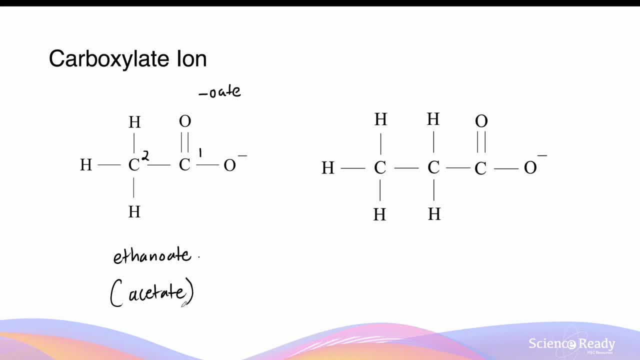 The other common name for ethanoate is acetate, which you may have come across already. Ethanoate is the IUPAC systematic name and this is the one you should be using for exams, whereas acetate is the name that you hear more commonly. There are 3 consecutive carbon atoms in this. 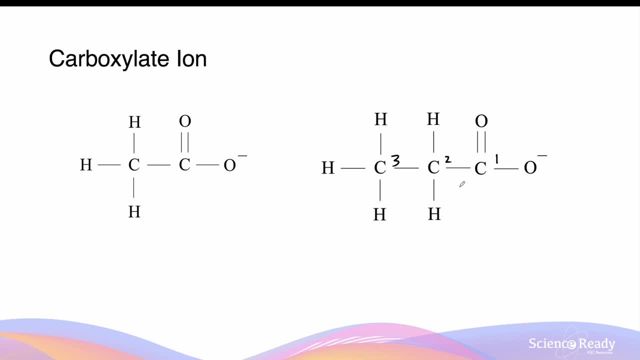 carboxylate ion. so the carboxylic acid used to produce it will be propanoic acid and the name of the carboxylate ion will be propanoate. It is very useful to know and remember that. 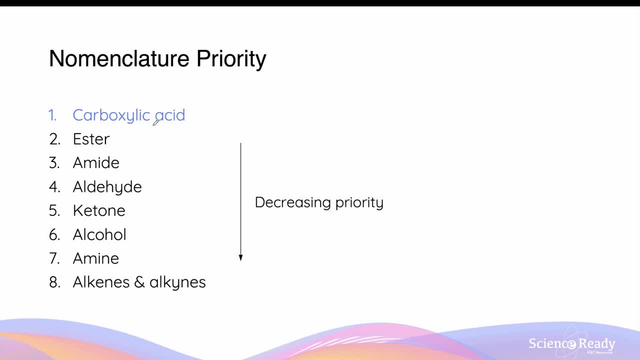 carboxylic acid has the highest priority out of all organic functional groups, which means that it has the highest priority out of all carboxylic acids, and that is why it is called carboxylic acid. If there are any other functional groups present in the carboxylic acid, they will be denoted. 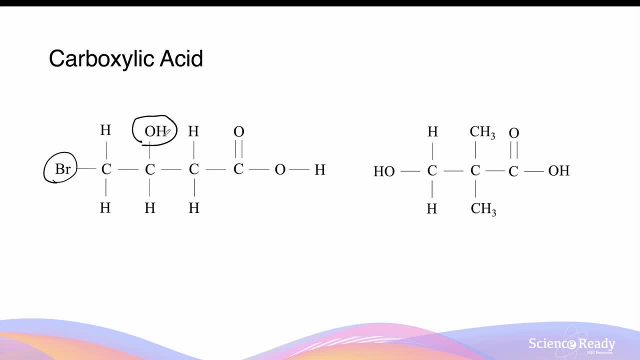 by the prefix, while the carboxylic acid will be denoted by the suffix. In a molecule where there is an alcohol and a bromine, both of these branches or functional groups will be denoted by their respective prefixes. so bromo for bromine and hydroxy for alcohol and the 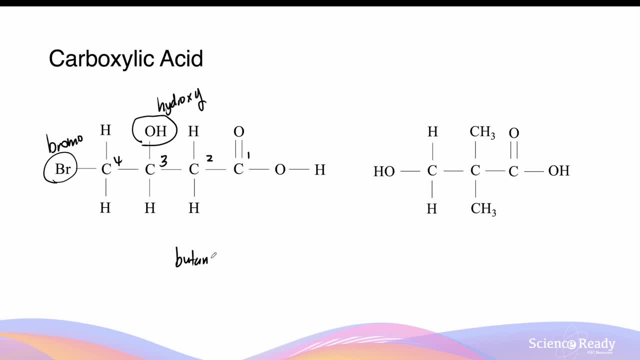 carboxylic acid will be left as its suffix, as usual. Therefore, the ending of this word is butanoic acid. Since B comes with a H, the bromo will be written first, so this will be 4-bromo 3-hydroxy-butanoic acid. 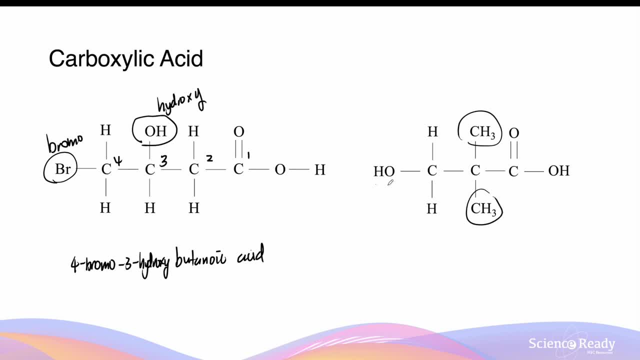 For the second molecule, again we've got methyl groups and alcohol, which will be all denoted as branches and prefixes, and the carboxylic acid will be again written as its suffix. So there are three consecutive carbon atoms. This is propanoic acid, so this will be 3-hydroxy. There are two methyl groups in the second. 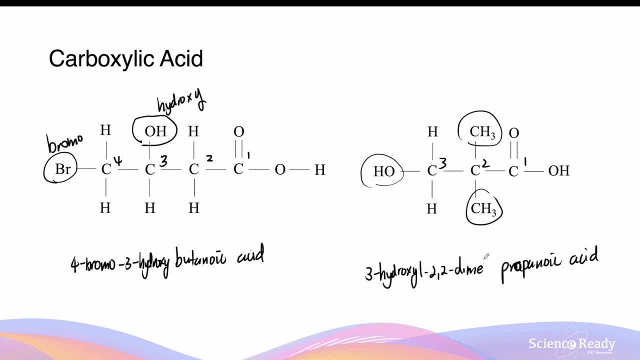 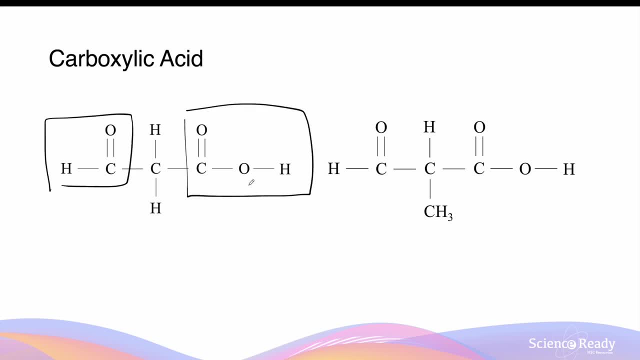 carbon, so this will be 2-dimethyl-propanoic acid. In this molecule there's an aldehyde functional group and there's also a carboxylic acid functional group If the aldehyde is at the other end of the molecule, opposite to the 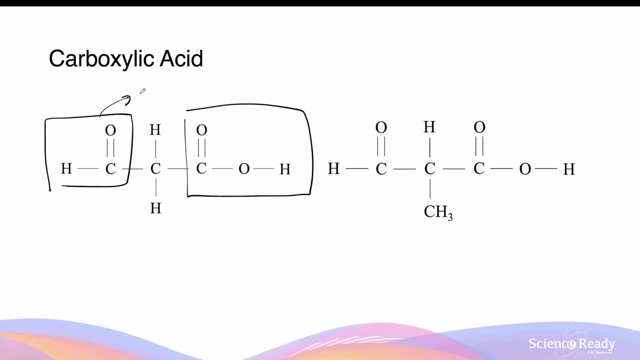 carboxylic acid. it's actually denoted by the prefix oxo, which is usually reserved for ketones. There are three consecutive carbon atoms. Number one is given to carboxylic acid because it has a higher priority than the aldehyde. 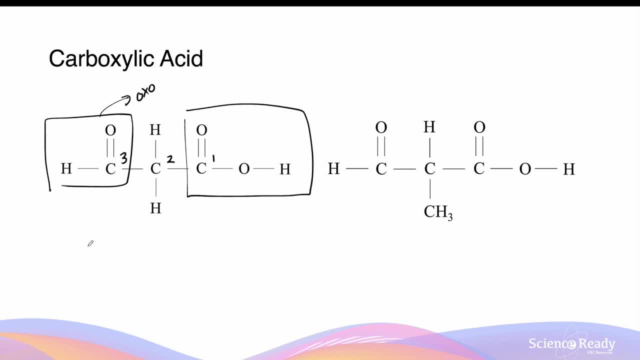 and therefore the aldehyde will be given the number three, So this molecule will be called 3-oxopropanoic acid. In the molecule on the right hand side we've added another carbon atom and hydrogen, to the metal carbon. In this case we actually count the carbon atom like this: where what? 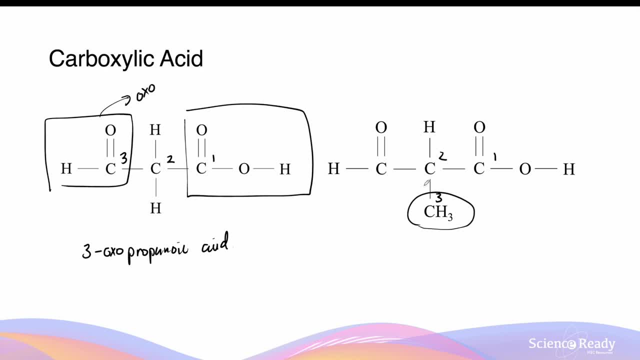 we've added is a molecule called 2-methyl-propanoic acid. This allows the aldehyde to become a branch which is denoted by the prefix of aldehyde formyl. Therefore, the name of this molecule is 2-formyl-propanoic acid. 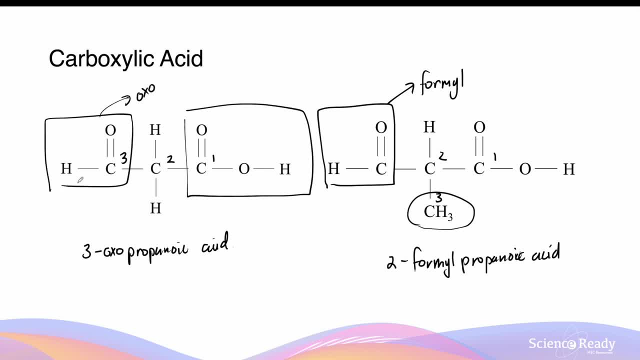 So you can compare the two molecules here. If the aldehyde is at the end of the carbon chain, we describe it using the prefix for a ketone, which is oxo. If we add the 2-methyl-propanoic acid, we can count the carbon chain such that the aldehyde becomes a branch rather than 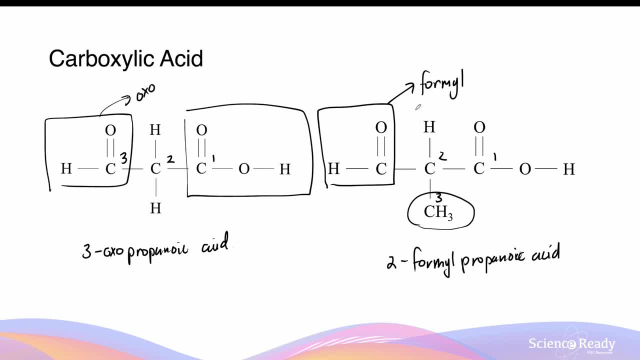 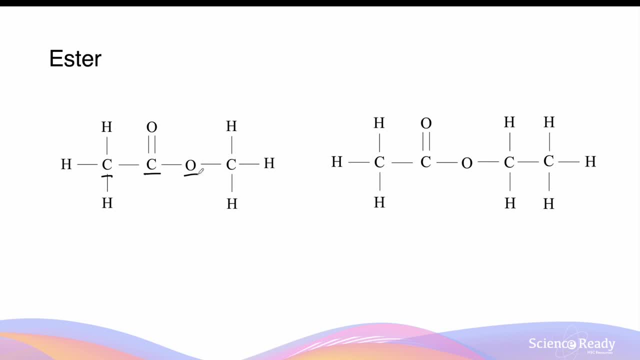 part of the main chain which is denoted using its usual prefix, which is formyl Esters, are carbonyl compounds, where the carbonyl carbon atom is next to a carbon atom, and oxygen, where the oxygen is further bonded to another carbon atom. 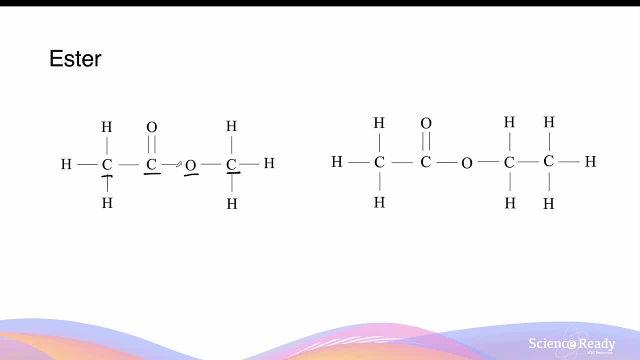 The name of the ester comes in two words or two parts. The first part is named by considering the carboxylate ion part of the ester. The carboxylate ion- part of the carboxylate ion is the conjugate base of carboxylic acids, so there are two carbon atoms in the ester. 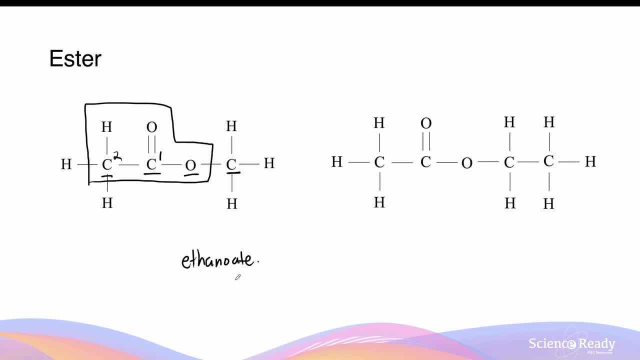 which means this will be called ethanoate. Attached to the ethanoate is one carbon and three hydrogens, which is similar to what we call a methyl group. Therefore, we will call this methyl ethanoate as two separate words with a space in between. 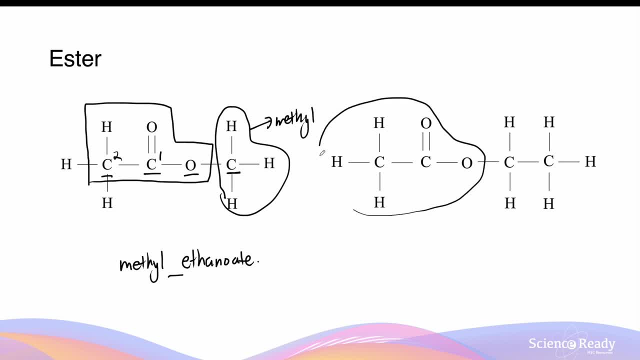 In this molecule. again, let's consider the carboxylate ion, part of the carboxylic acid In this molecule. we will consider the carboxylic acid. Once we know the carboxylic acid, we also know the methyl Goo six molecule when we interleave. 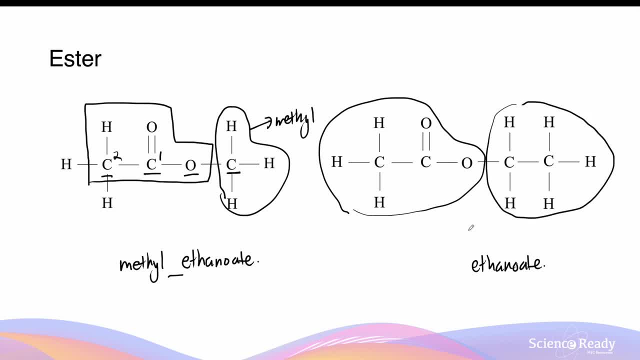 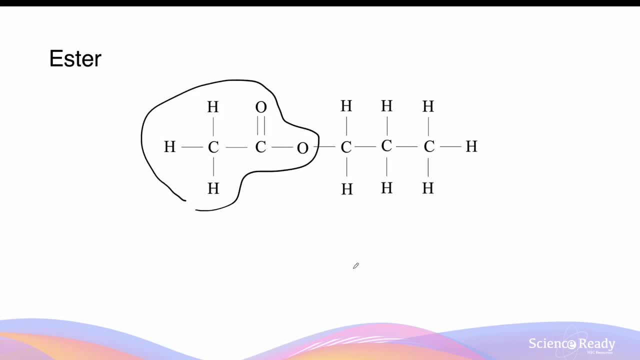 the phosphorous. So we first have to hot retired the methyl Goo six molecule, and so we will need to У1 result, an ester in the same functional group. the ester will be named according to its prefix. In other cases, where the ester is combined with anything below this list, the ester will take its. 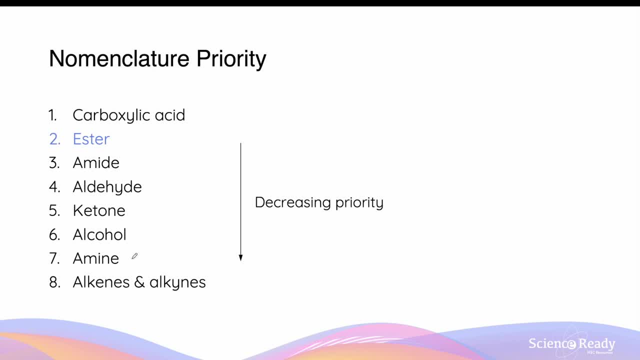 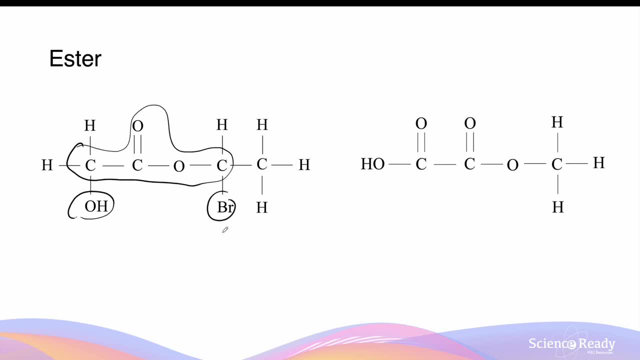 usual name, while the other functional groups will be denoted by the prefixes respectively. In this molecule there's an alcohol, an ester functional group and a bromine. Since esters have higher priority than alcohols, we'll name this according to the normal name of the ester. 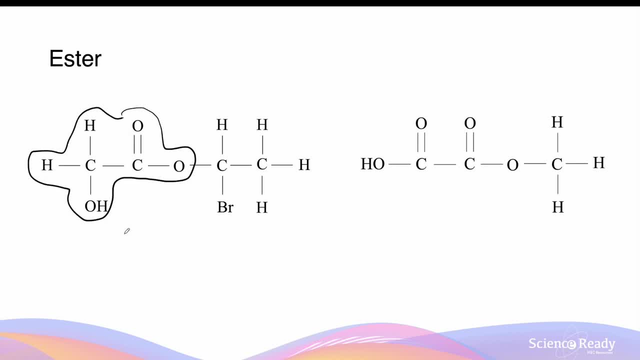 First of all, the carboxylate part here has two carbons, so we'll name this as ethanoate, as usual Here. since we have an alcohol attached to the second carbon of the ethanoate, we'll name this as two hydroxy ethanoates. There are two other carbon atoms on the 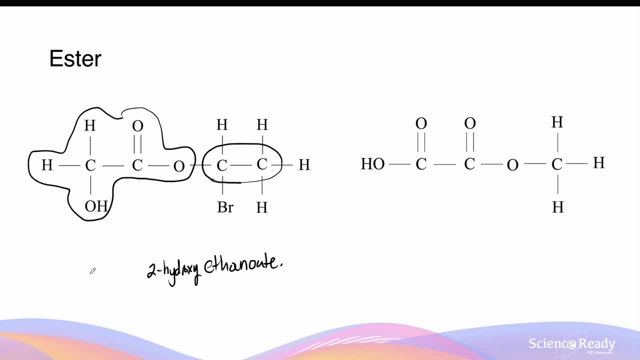 other side of the oxygen in the ester, and this is normally named as ethyl, and the bromine atom is on the other side of the oxygen in the ester, and this is normally named as ether, the first carbon of the ethyl group. so we'll call this 1-bromo-ethyl-space-2-hydroxyethanoate. 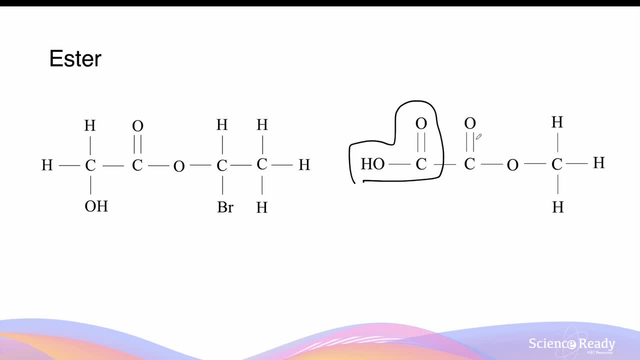 In this molecule there's a carboxylic acid which has a higher priority than the ester on the other side of the molecule. This means the carboxylic acid will receive a suffix and there's only one carbon. so therefore this is methanoic acid. This carbon atom is 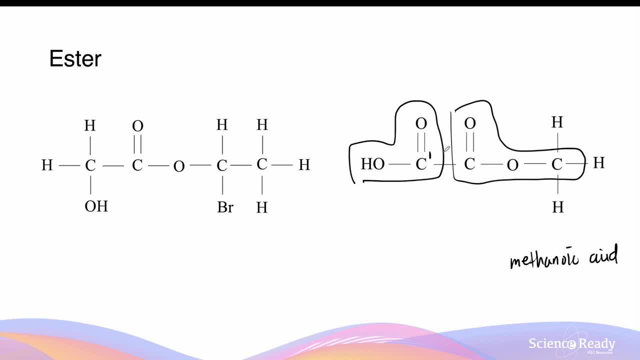 not included in the main carbon chain because it is part of the ester branch. The prefix of an ester is generally described as alkoxy-carbonyl, where the carbonyl denotes the carbonyl carbon and alkoxy describes the number of carbons on the other side of. 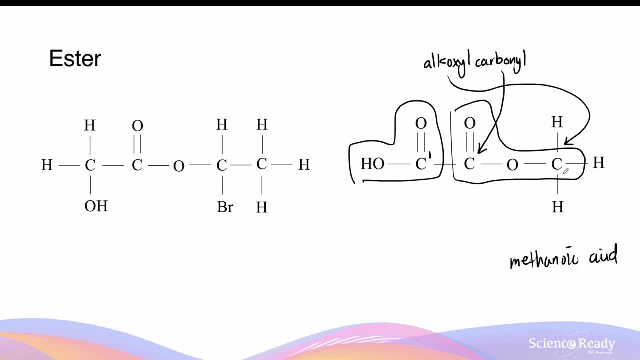 the oxygen. In this case there's only one carbon atom, so therefore this is called methoxy-carbonyl. The methoxy-carbonyl, which is the ester, is bound to the first carbon of the methanol methanoic acid, so we'll name this as methoxy-carbonyl methanoic acid. We do not need to number the 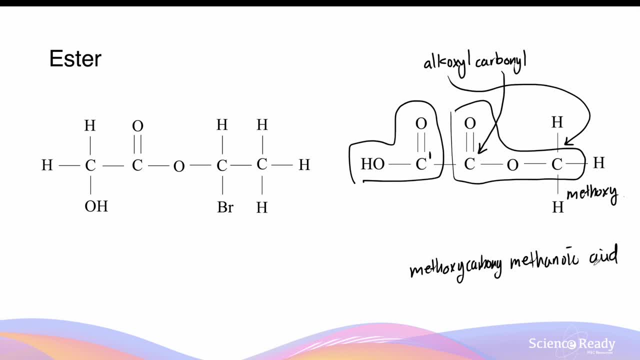 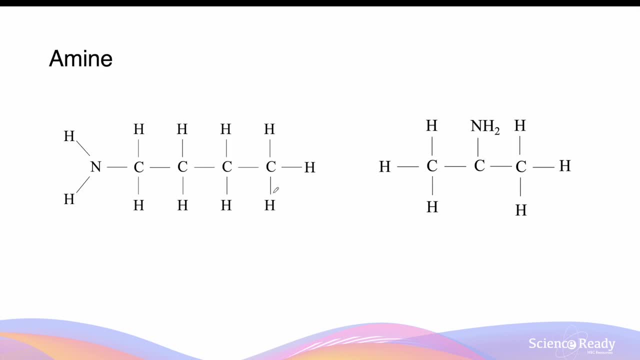 methoxy-carbonyl, because there's only one carbon on the methanoic acid. If there were more carbon atoms, you would need to write a number in front of the ester branch. Amines are molecules where a nitrogen atom is connected to a carbon atom that has single. 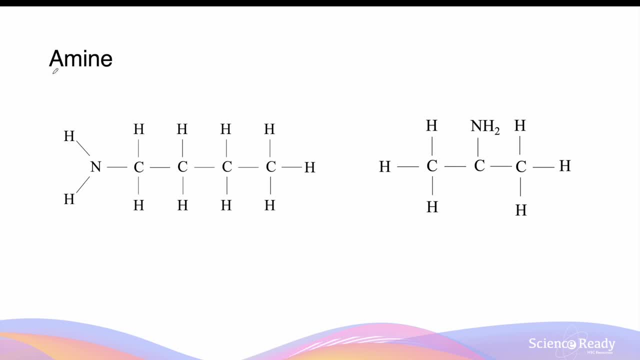 bonds only. The suffix of amines is easy because it literally ends with amine. In this molecule there are four consecutive carbon atoms and an amine functional group of the nitrogen atom is bonded to the first carbon. Therefore the name of this molecule is butane for four, one amine. 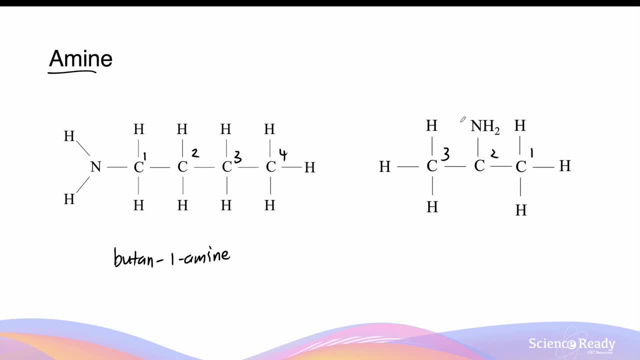 In this molecule there are three consecutive carbon atoms and the amine group is on the second carbon, so this is called propan-2-amine. These two amine molecules are classified as primary amines- amines because the nitrogen atom is only bonded to one carbon atom, So you can see one carbon atom. 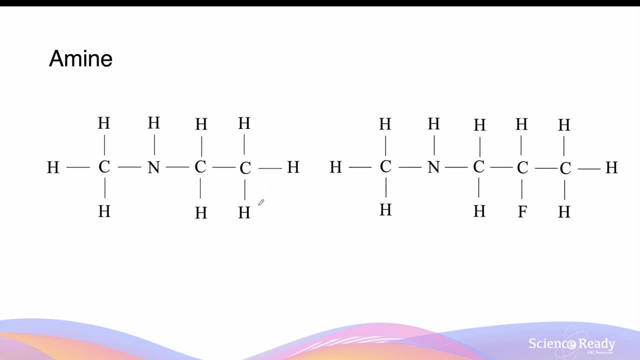 one carbon atom. In other cases, nitrogen atoms can be bonded to more than one carbon. In this case, the nitrogen atom is bonded to two other carbon atoms, two other carbon atoms, and these are therefore described as secondary amines. The naming of secondary amines are different to. 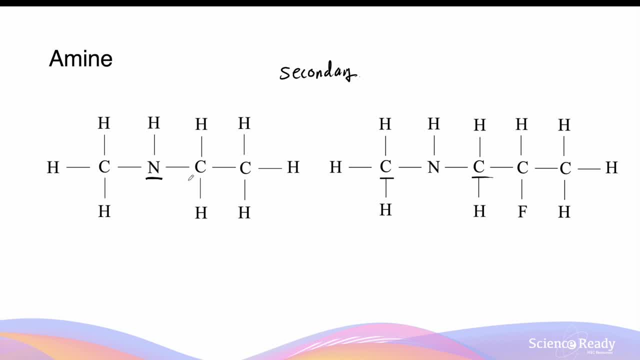 primary amines. First we need to identify what's the greatest number of carbon atoms. consecutively, that contains the amine functional group. In this case there's two, So the suffix of this name will be ethane, amine or ethanamine. The remaining carbon will become a branch. 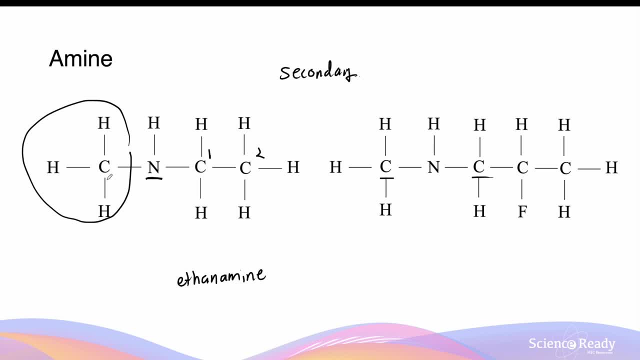 so in this case this is a methyl group. The methyl group is connected to a nitrogen atom, so we'll denote this using the letter N instead of any numbers: N-methyl-ethanamine. In this molecule there is one, two, three consecutive carbon atoms that 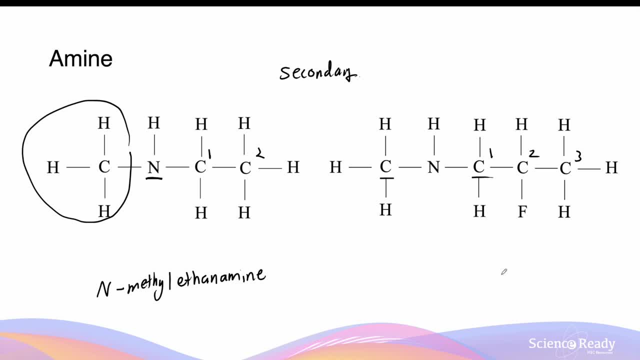 contains the amine functional group. Therefore the ending of this name will be pro-panamine or propanamine. The methyl group is again on the nitrogen atom, so we'll call this N-methyl- propanamine. In addition, there's another fluorine atom on the second carbon atom. 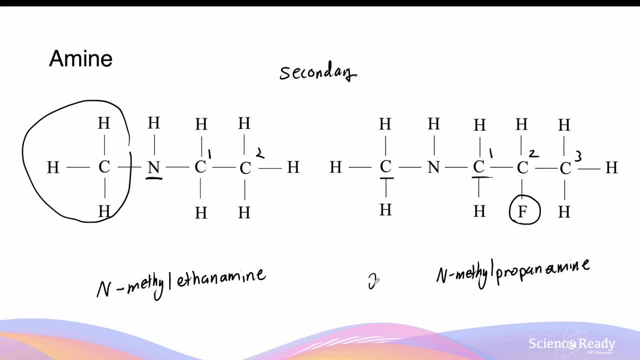 carbon of the propanamine, so we can easily describe as 2-fluoro-n-methyl-propanamine. Notice how I've written the fluorine before the methyl, because F comes with an M in the alphabet. A tertiary amine is where the nitrogen atom is bonded to carbon atoms. only there are 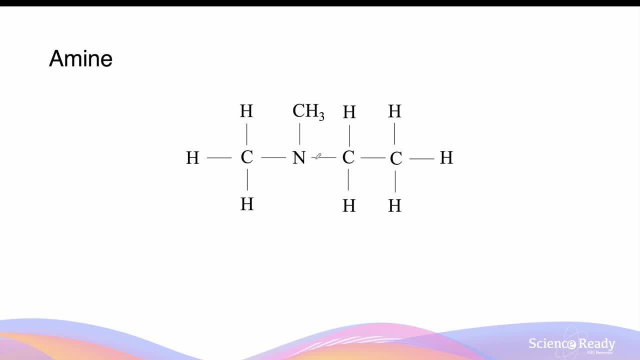 no hydrogen atoms. The naming of tertiary amine follows the same rule as secondary amines. First, we identify the carbon chain that has the greatest number of consecutive carbons. there's two here, so we'll write this as ethanamine. 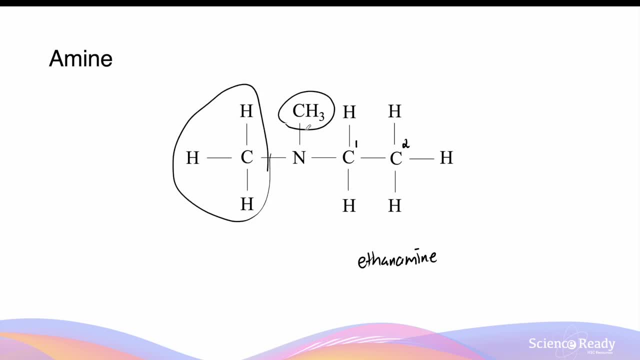 The remaining carbon atoms, that's bonded to a nitrogen, become branches again. Now there are two methyl groups here, so we'll write this as n-n-dimethyl-ethanamine. This is a tertiary amine. What about this example? Amines have relatively low priority compared to other functional groups. 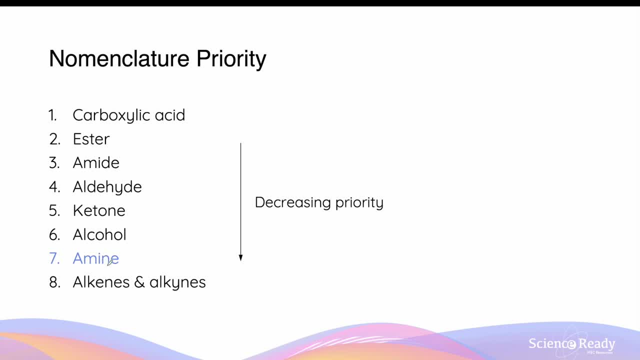 They are more important than alkanes and alkynes, but less important than every other functional group. So in most cases amines, when combined with other functional groups, will be denoted by the prefixes instead. The prefix for amine is amino. 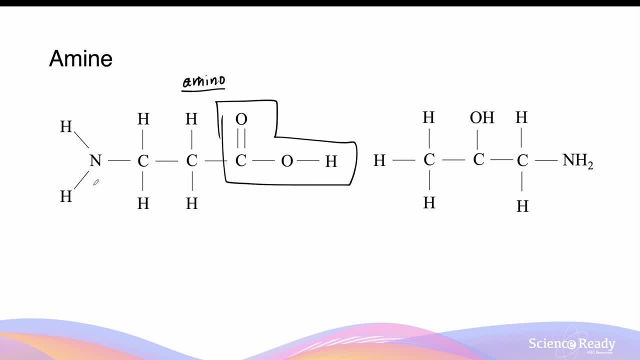 So in this molecule, where you have a carboxylic acid, which has the highest priority, and an amine, this will be called 3-amino, because the amine is attached to the third carbon, propanoic acid. In this molecule there's an alcohol and an amine. 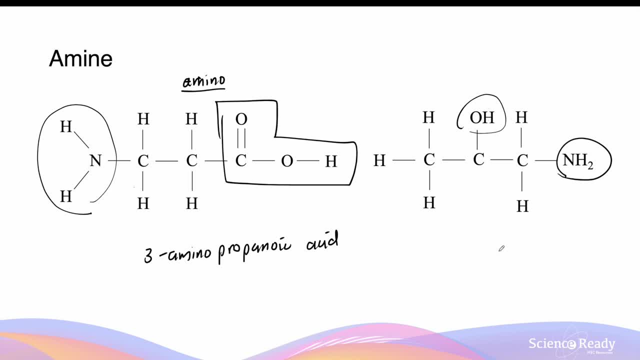 Alcohol has higher priority than amines, So this will be called propan-2-ol, where the suffix is for the alcohol. If we count the molecule from right to left- 1,, 2,, 3,- the amine will be on the first carbon. 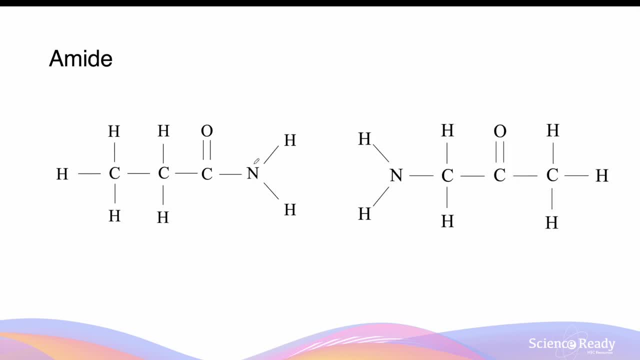 So this is 1-amino-propan-2-ol. Amines are carbonyl compounds where the carbonyl carbon is next to a carbon atom and a nitrogen atom. For amide, the nitrogen atom must be right next to the carbonyl carbon. 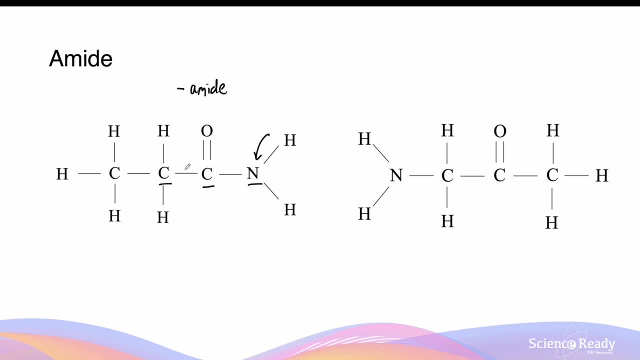 The suffix for amide is its own name, which is amide. In this molecule there are three consecutive carbons containing the amide functional group, so therefore this is called propanamide If the nitrogen atom is only bonded to the carbonyl carbon and two other hydrogens and 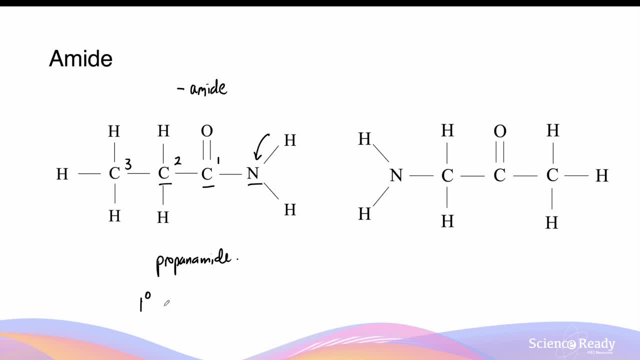 no other carbons. this is what we describe as a primary amide. The categorised primary, secondary and tertiary amide is exactly the same as for amines. This molecule on the right hand side may seem to be amide, but it's actually not, because 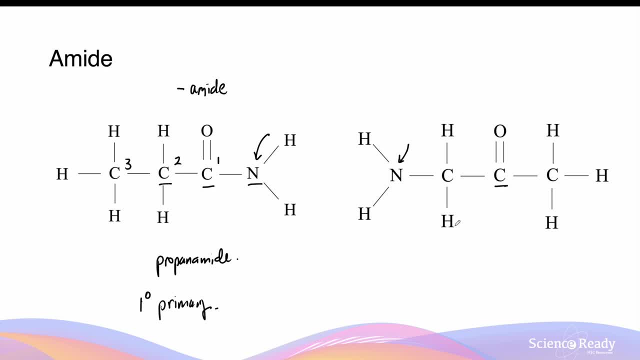 the nitrogen atom is not next to the carbonyl carbon. In this molecule there's actually an amine group and a ketone functional group, Since the ketone has a higher naming priority compared to the amine. the name of this molecule. 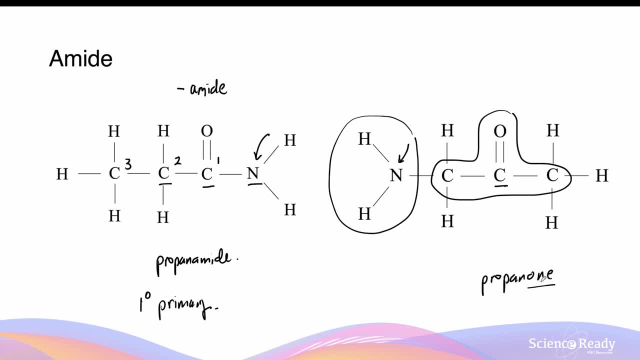 is propanone, where O and E is the suffix for ketone And the amine group is on the first carbon. this is called 1-amino-propanolone When the amide nitrogen atom is bonded to another carbon atom in addition to the carbonyl. 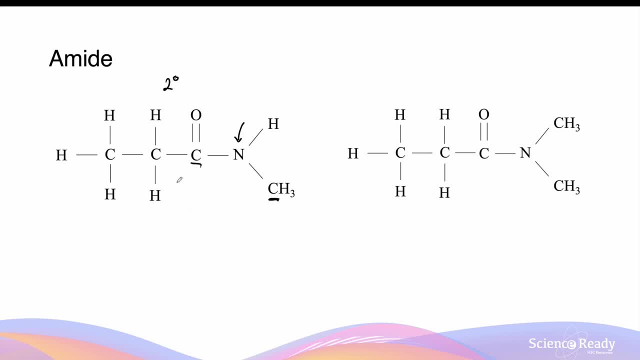 carbon. this is what we call a secondary amide. In a secondary amide, we still start counting the carbon chain that has the greatest number of carbon atoms, and of course the first carbon is always the one that has the carbonyl group. 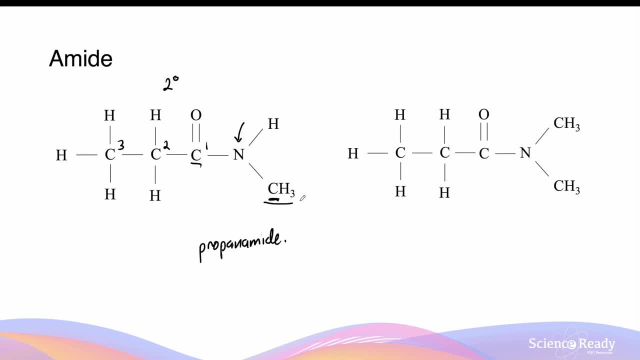 This is called propanamide. once again, The leftover carbon atom and its hydrogens becomes a methyl branch, which is connected to the nitrogen atom, so this is written as N-methylpropanamide. If the nitrogen atom is bonded to two additional carbon atoms on top of the carbonyl carbon, 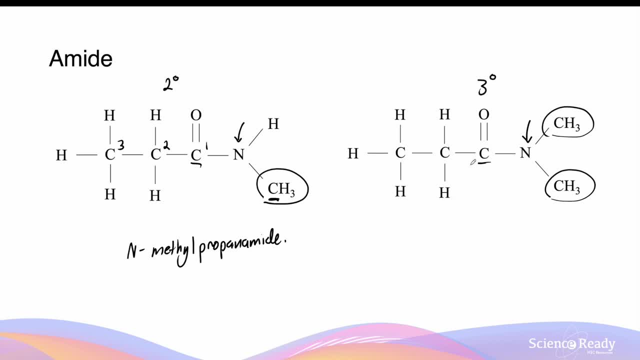 this is what we call a tertiary amide. The name of this tertiary amide also ends with propanamide, because there are three consecutive carbon atoms. The remaining two carbon atoms are two separate methyl groups. both are attached to the nitrogen, so this is called NN-dimethylpropanamide. 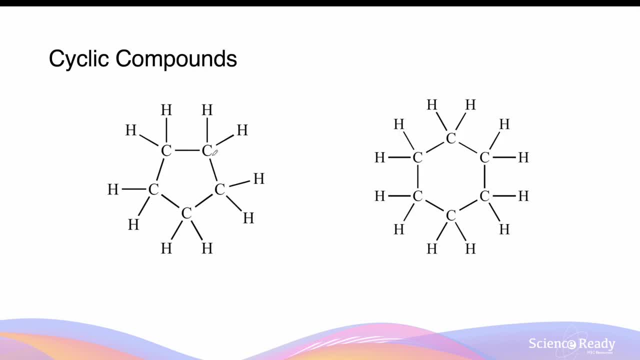 Cyclic compounds are organic molecules where the main carbon chain forms a ring shape. The name of cyclic compounds contain the prefix cyclo. For example, in this molecule where there are five consecutive carbon atoms in a ring shape, this is called cyclopentane. 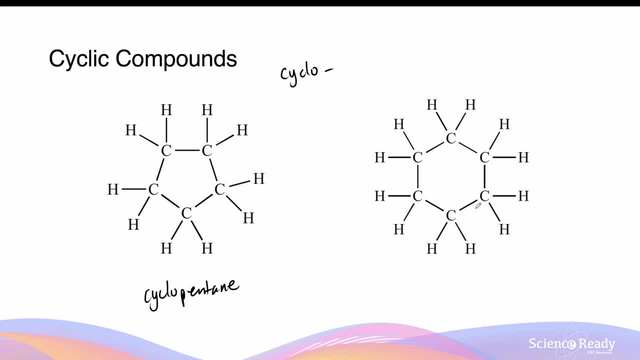 In a cyclic compound with six carbons, where this is also an alkane with only single carbon-to-carbon bonds. this is called cyclohexane. Cyclic compounds can also contain functional groups such as alkynes and alcohols. The name of this compound is cyclohexene. 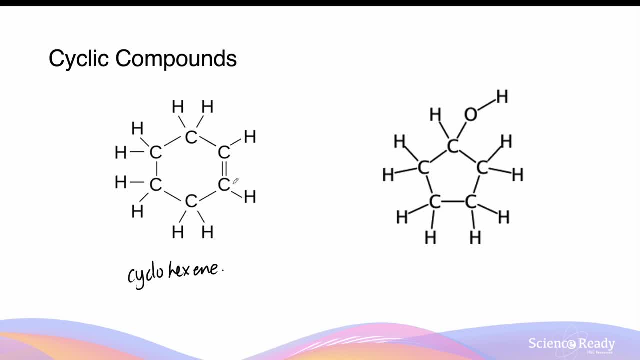 In a cyclic molecule, we do not need to use numbers to denote the position of the alkyne functional group, because it is presumed that the alkyne bond lies in the first bond position. Similarly, for alcohols, The position of the alcohol functional group is presumed to be on the first carbon atom. 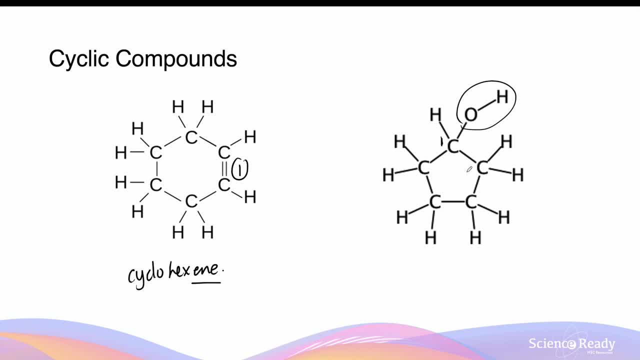 and therefore in the name of this molecule we do not need to use numbers to denote its position. The name of this molecule is cyclopentanol. In this molecule of cyclohexene there's a bromine atom situated on one of the other. 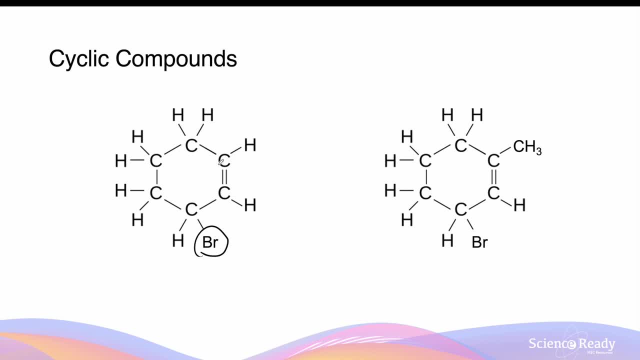 carbon atoms. Again, we presume that the double bond lies in the first bond position. So we'll count from the first carbon here, 2,3,4,5,6.. So there are again six carbon atoms in the ring structure, which means the name of the. 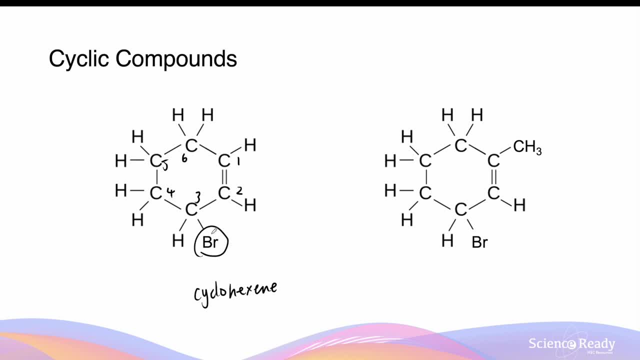 molecule will be cyclohexene. The bromine atom, when counted this way, will be attached to the third carbon atom, So this will be 3-bromo-cyclohexene. Note that I've decided to count the number of carbon atoms in a clockwise manner rather. 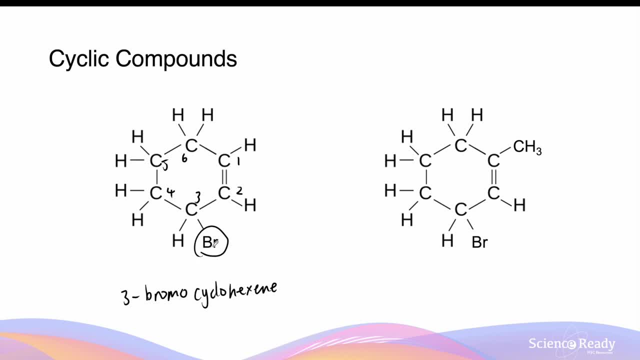 than anticlockwise, because this way the bromine substituent will be on the third carbon rather than the fifth carbon. So Here the alkene functional group will always receive the number one bond position. You will need to think about the direction of counting the carbon atoms in a cyclic compound. 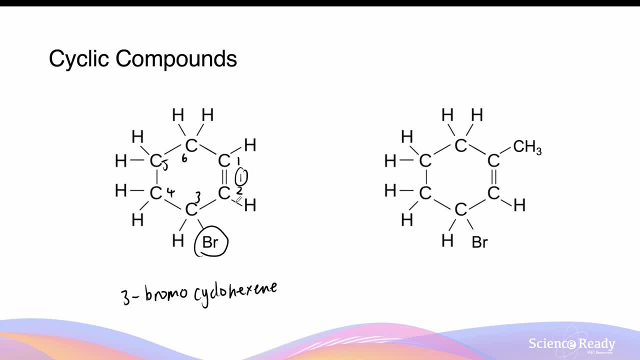 You will choose the direction that will give you the lower number for any of the other atoms or branches attached to the cyclic molecule. In this case, besides the bromine atom, we also have a methyl group. We again will count the carbon chain, starting with the same carbon atom. 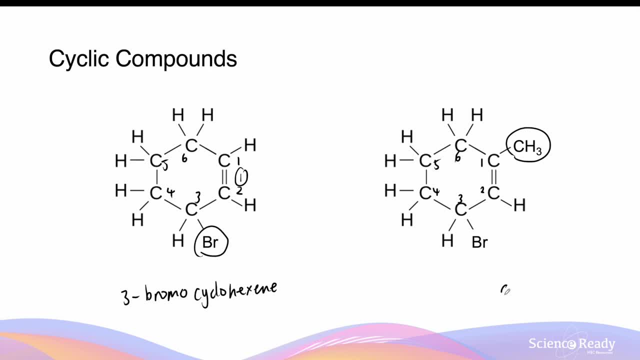 So there are again six carbon atoms. The name of this molecule will end with cyclohexene. The methyl group is now on the first carbon and the bromine is again on the third carbon. We'll write the bromine in the name first, 3-bromo, because the letter B comes before. 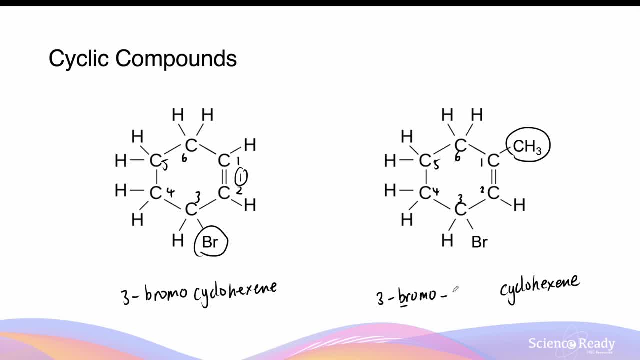 the letter M in methyl in the alphabet 3-bromo 1-methyl cyclohexene. Again, notice how I haven't written any numbers for the alkene double bond, because it is presumed by convention that it is in the first bond position.